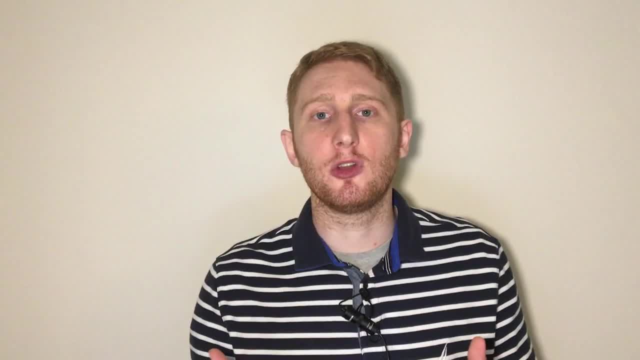 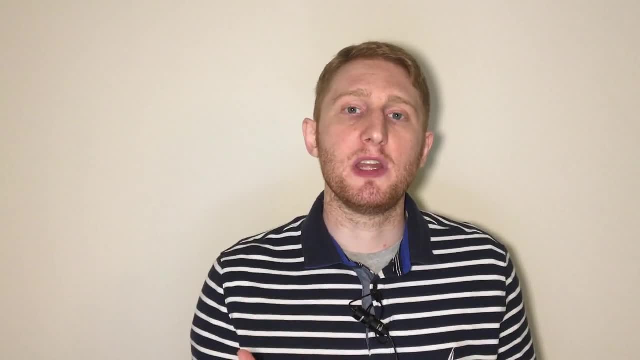 through the Language Arts extended response section for those who don't really have a clue where to start, or those who have never been good writers before but now need to ace the GED Language Arts section. So what I'm going to give you in this video is a step-by-step approach that 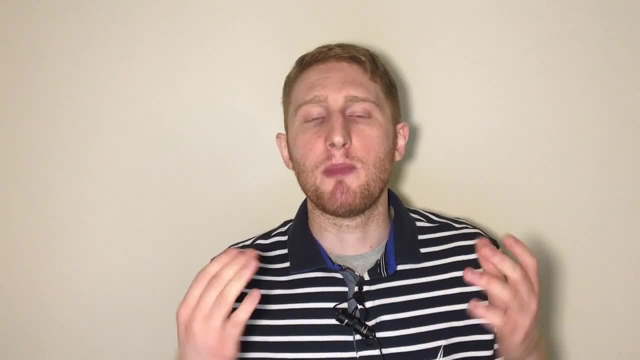 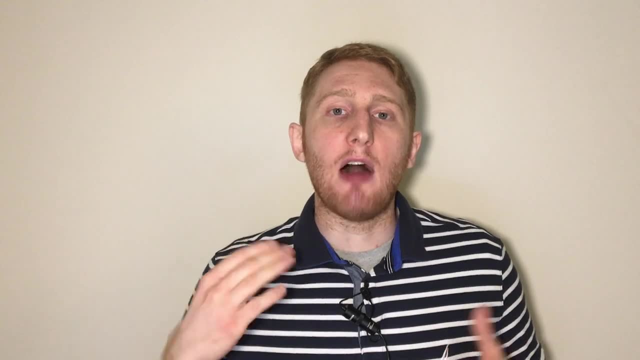 you can use to maximize your score on the essay. We're going to try to help you minimize the pain of writing here, and I'm going to go over things like how long you'll have to write how many words and how long your essay should be, as well as what the essay should be about. I'm also going to give 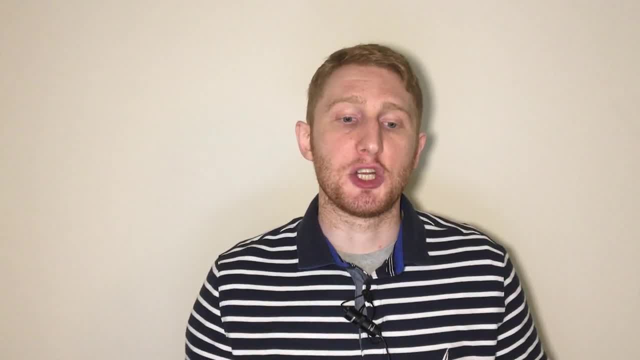 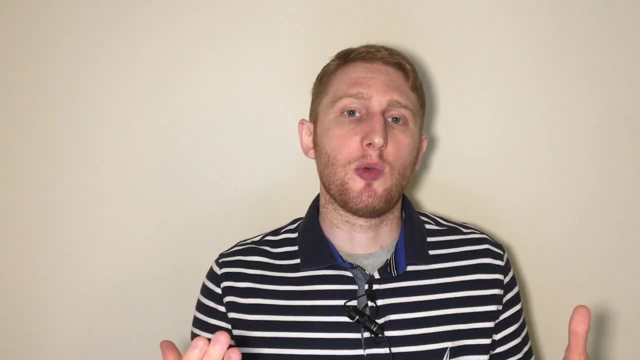 you a basic formula that you can use to easily ace the essay section, and we're also going to look at some specific examples together, and I'm going to throw out many other great tips and tricks and strategies along the way. So let's get started. So, as we go through the video, please note that 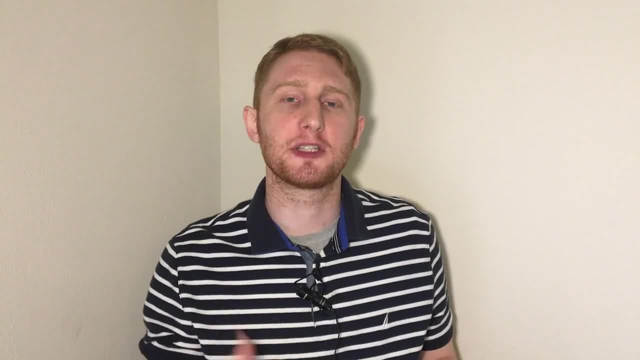 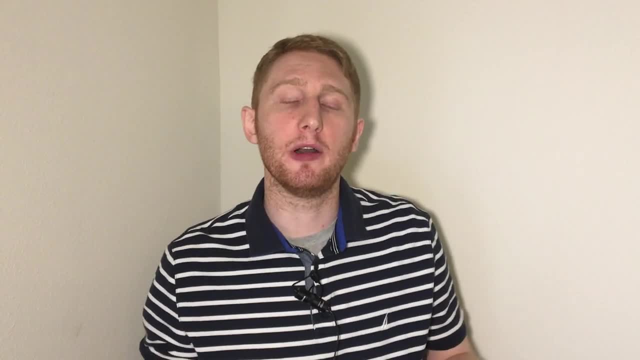 different people call the section different things, So let's get started. Some call it the Language Arts extended response, some people call it the extended response essay and some people just call it the GED essay. And throughout the video I'm probably going to call 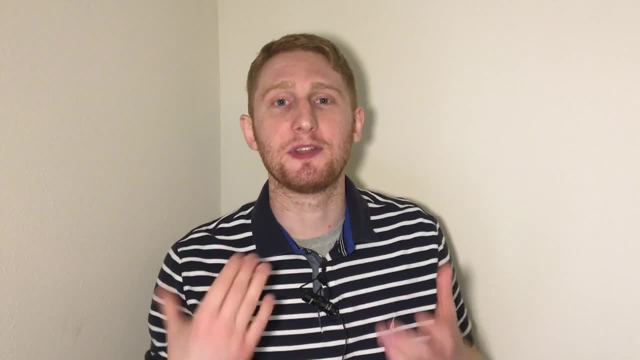 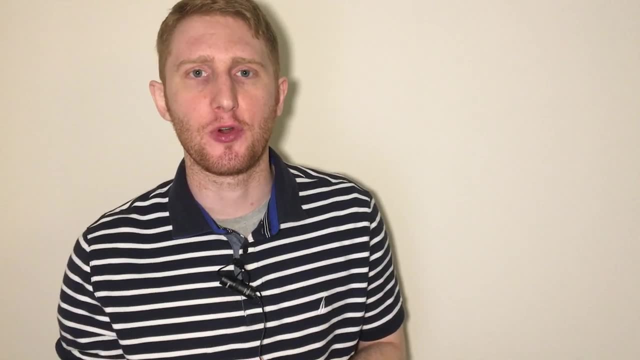 it by each of these different names, so just be aware that I'm talking about the same thing here. The GED essay is a major source of stress for many test takers, but how much does it really impact your score? Here's a valuable insight we get from a GED test teacher in Colorado with the 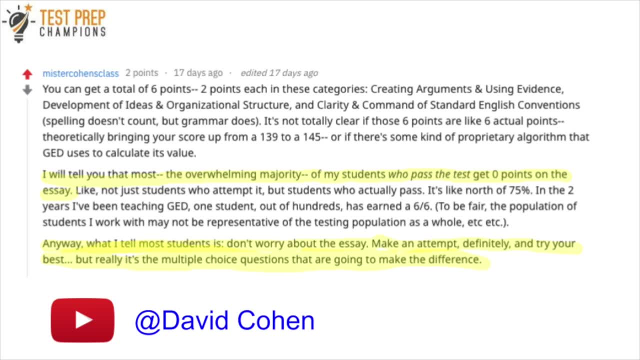 Reddit username MrCohensClass, and this is right off of Reddit. He says: I will tell you, the overwhelming majority of my students who pass the test get zero points on the essay. And he tells most students: don't worry about the essay. 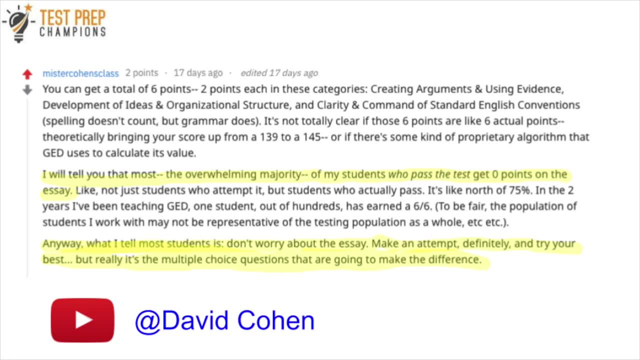 make an attempt, definitely, and try your best, but it's really the multiple choice questions that are going to make the difference, And you can find him on Reddit, MrCohensClass, or on YouTube. The YouTube username is David Cohen. He's got an amazing channel with some really brilliant content. 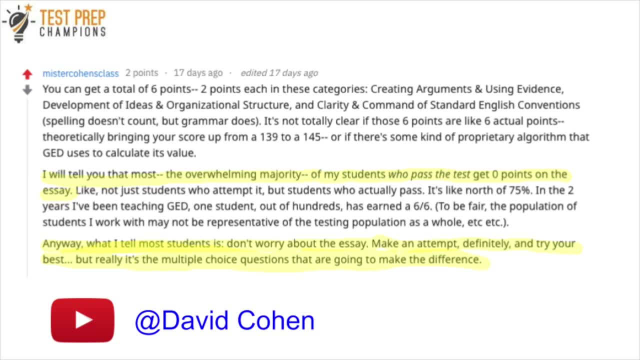 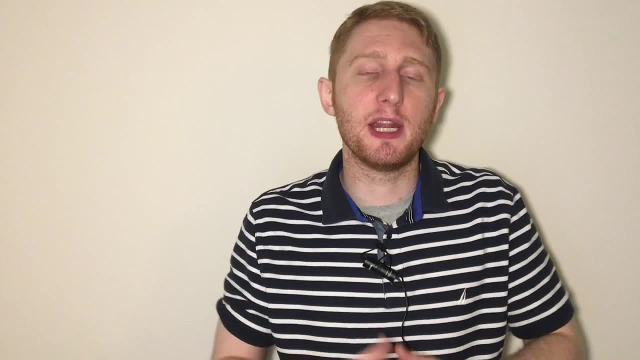 to help you pass, I highly recommend subscribing to David Cohen's YouTube channel. I'll link to that down below and you can also search him on YouTube. The key point here is not to stress too much about the essay, because if you completely vomit as long as you've done really well on the 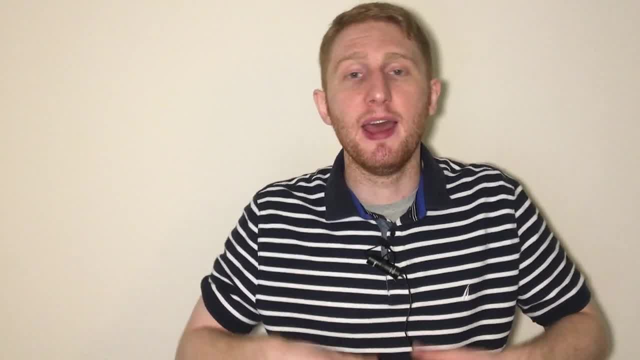 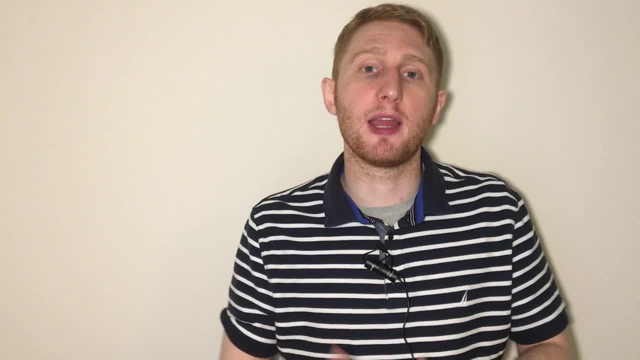 multiple choice portion. there's still a really good chance that you can pass. But that being said, you know I really want you to prepare anyway for this, because you don't want to waste your time and you don't want to waste your money. You really want to go in there and be aggressive and go after all. 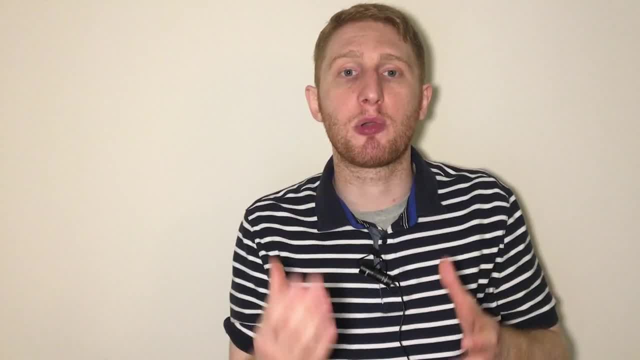 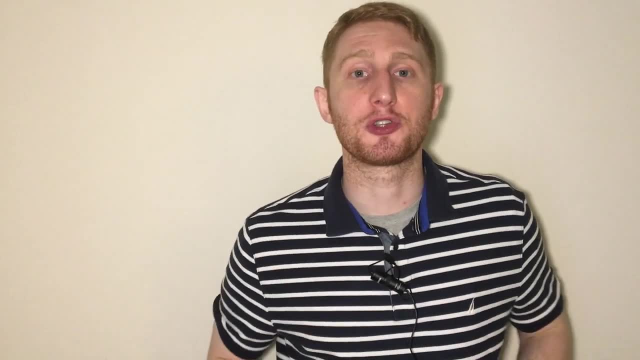 the points you can and not leave points on the table for the essay. So I'm going to give you an approach here and the rest of the video And if you use it, you should be in good shape for the essay here. But, like I said, don't stress it too much. It is just a small portion of your score. 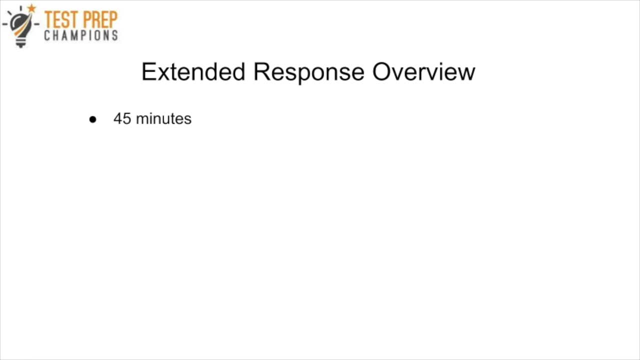 Now let's look at an overview of the extended response section. You're going to have 45 minutes in total to write your essay, and don't worry about it. You're going to have 45 minutes to write your essay. Don't worry, because I'm going to show you how to budget your time. in just a minute. A good essay. 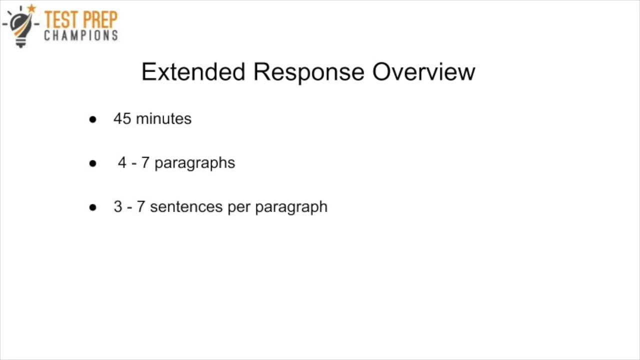 should have between four to seven paragraphs and three to seven sentences per paragraph. 70 to 80 words per paragraph is a good amount to shoot for, And this would come out to a total of 300 to 500 words. Now, some of you might be panicking a little bit, but I just want to. 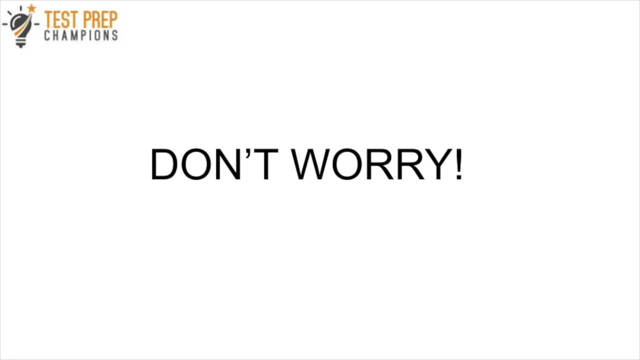 remind you. please don't worry, Absolutely don't worry. We're going to go over what all of this means: Paragraph sentences, word counts- It's nothing to stress about. I'm going to go over this and I'm going to give you that approach. I just wanted to introduce the extended response. 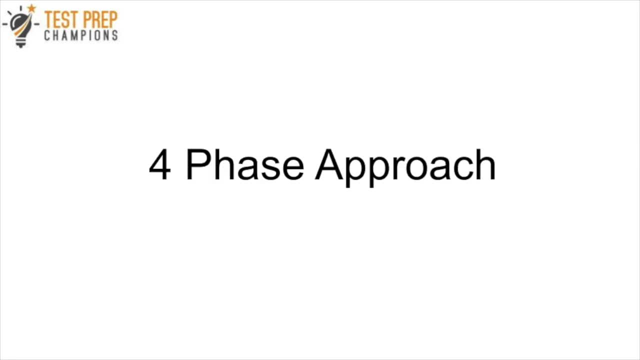 overview here. To write your essay, I recommend the following four phase approach. First, you're going to read the two passages that you're presented with and then you're going to come up with a plan And I'm going to give you some things to look for as you're reading, so you can. 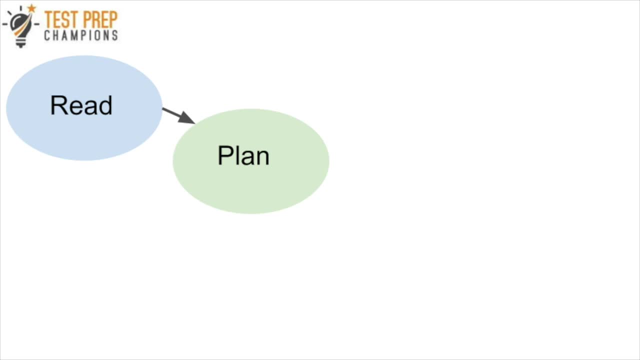 start your plan while you're reading, And really the planning step is probably the most important step here, because you've got a good plan which I'm going to show you how to make. Then your writing should just flow naturally and easily from the plan. So the third phase is the actual writing. 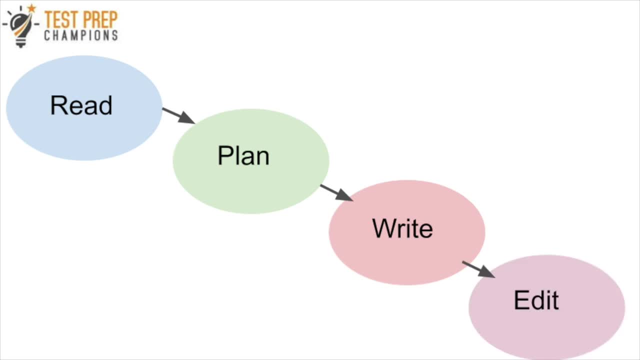 and that's going to take up most of your time, And whatever time you have left is going to be editing your essay for things like clarity and grammar and making sure that your sentences have a logical flow to them, Having a strategy to budget your time while you're writing your essay. 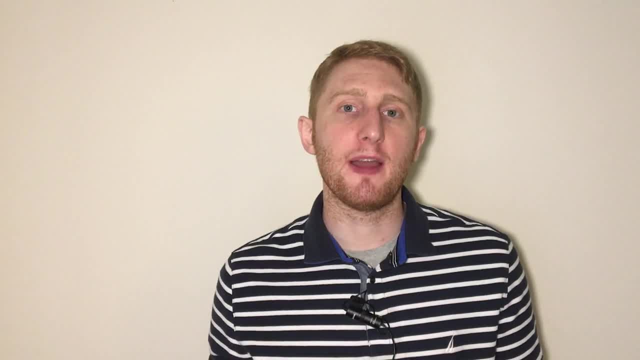 is very, very important. As I said earlier, you'll have 45 minutes in total to write the essay, But how do you divide your time up? Well, that's what I'm going to show you. next, I'm going to give you. 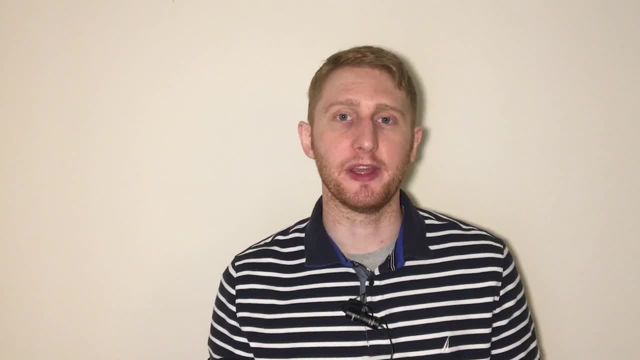 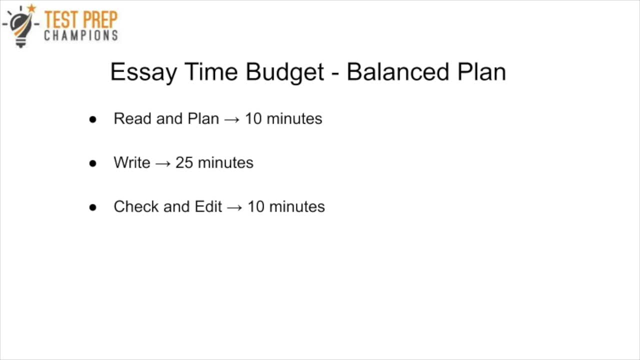 a couple of different strategies and you can pick whichever one you think is going to work best for you. The first way of budgeting your time is what I call the balance plan, And it's the most balanced plan. So you'll budget 10 minutes to read and plan 25 minutes to write, and then 10 minutes. 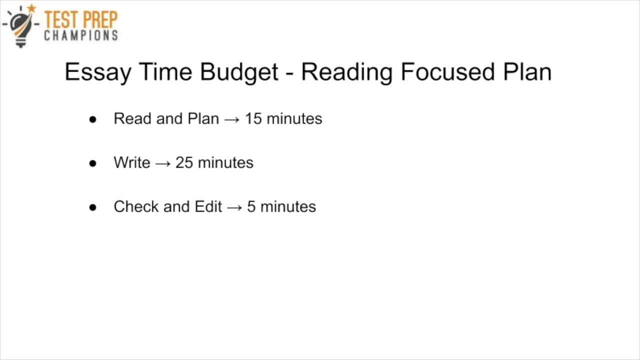 to check and edit your work. Now you can also do a reading focus plan, which gives you a little bit less time to check and edit, but more time for reading and planning. So you would budget 15 minutes to read and plan, 25 minutes to write and then five to check and edit. Now, if you want to, 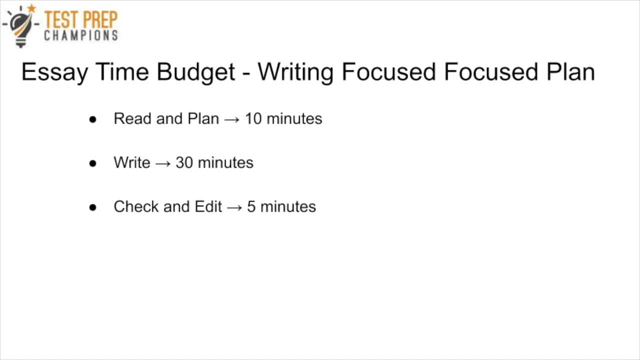 maximize the amount of time to write, then I'd recommend you go with the writing focus plan, which has you budgeting 10 minutes to read and plan 30 minutes to write and then five to check and edit. Now again, the general theme here is: do not worry, Don't worry, You don't have to make a 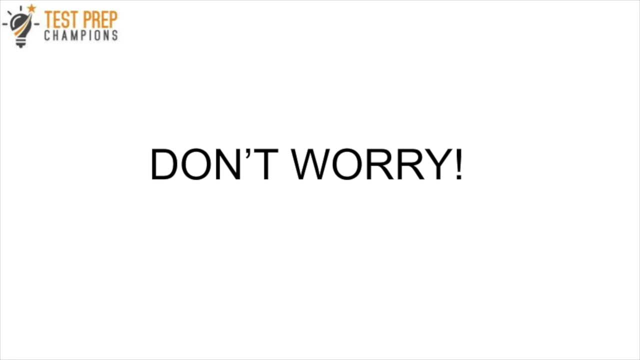 decision and commit to it 100%. I just want you to understand that these are general strategies and frameworks that you can use. You don't have to follow one of these plans exactly to the T. I just want you to have some kind of strategy so that when you're sitting there trying to write, 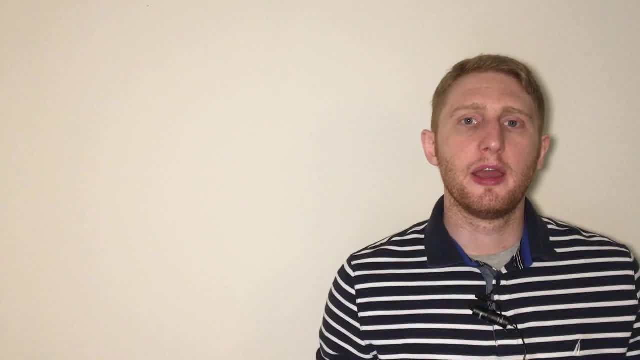 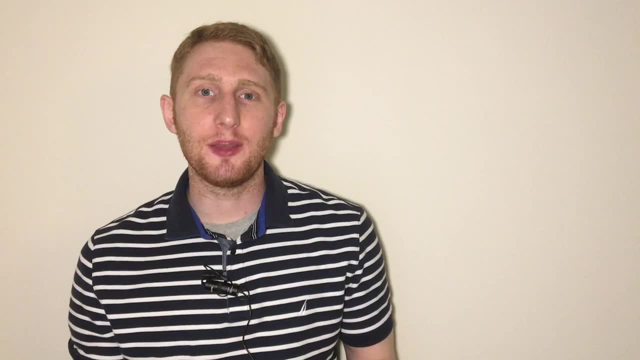 your essay and the timer's clicking down, you don't panic. Next, let's move on and let's talk about the prompt that you're going to be asked to write about. So let's start with the prompt that you're going to be asked to write about for your essay. While it's impossible to know exactly what, 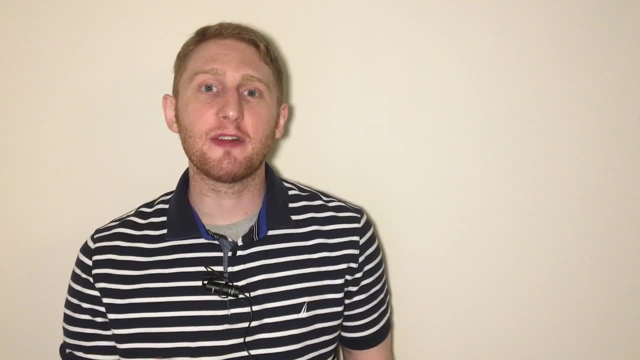 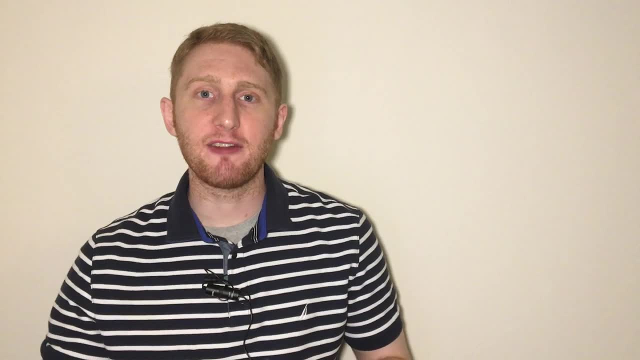 the topic is going to be. we do know that you're going to be given two different passages written by two different authors. Each author is going to be trying to make an argument and you're going to have to identify the arguments of both authors and identify who is making the stronger argument in 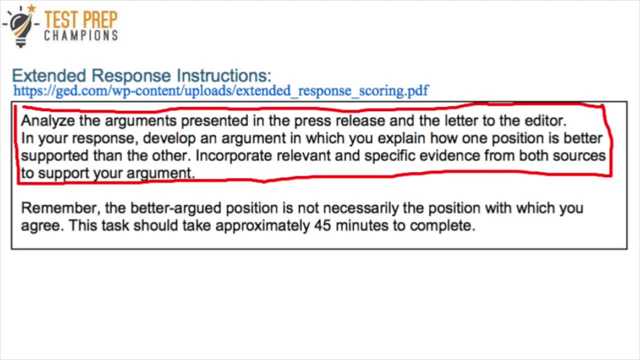 your essay. Let me show you an example, and this comes from an extended response prompt and the prompt says: analyze the arguments presented in the press release and the letter to the editor. Any response to the argument is not a strong argument. If you're trying to make an argument, 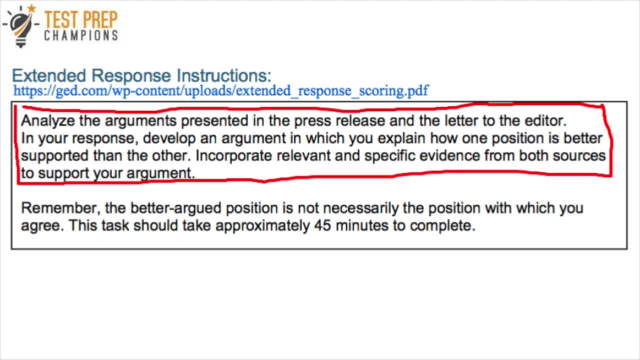 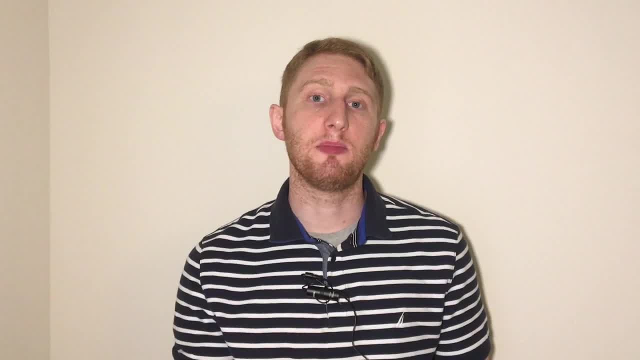 you're going to want to develop an argument in which you explain how one position is better supported than the other and incorporate relevant and specific evidence from both sources to support your argument. This prompt is an example of a typical prompt that you're going to get on the GED. 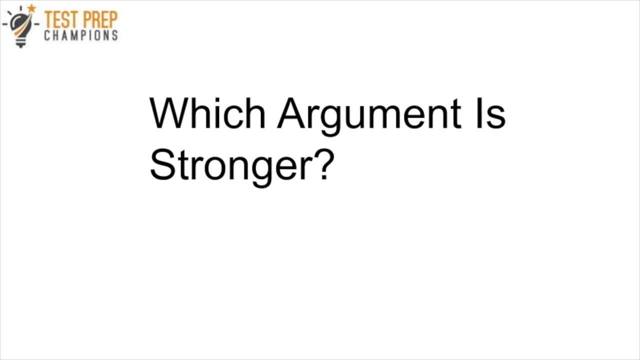 test. Okay, this segment is very important here, So when it comes time to trying to decide which author is making the stronger argument, there are several factors to consider here. So strong arguments include specific examples rather than vague examples, and they're not going to be. 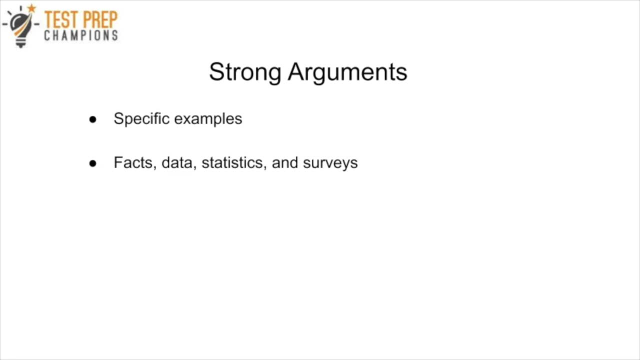 specific examples, and they also include facts, data, statistics and surveys to back up their claim. They may also quote or reference experts and authority figures who have an opinion on the topic. Strong arguments also will include recent dates, So a survey from, let's say, a couple years. 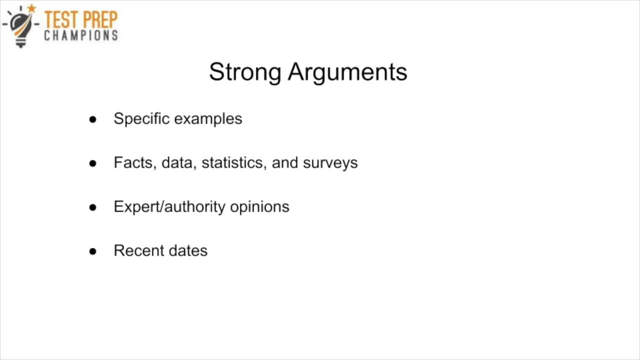 ago is probably going to be more credible than something that happened maybe 50 years ago. generally speaking, of course, Okay, and so also results from research. studies and experiments are also big signs that someone is making a compelling and credible argument. What are some signs of a weaker argument? Well, first of all, 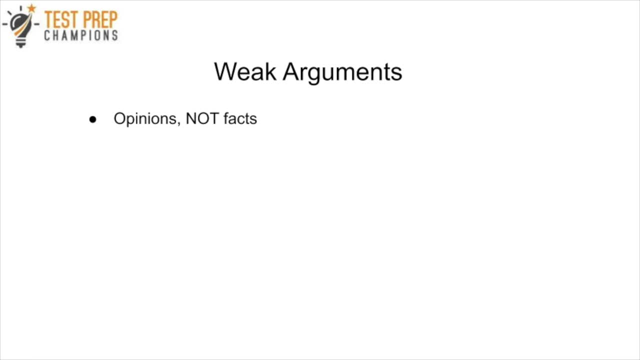 when someone uses an opinion or a lot of opinions, but not facts, that's usually a sign of a weaker argument. Now, this can vary. if it's an expert's opinion- Like, for example, if it's a health topic and a doctor is sharing their opinion or a different authority figure, then the opinion 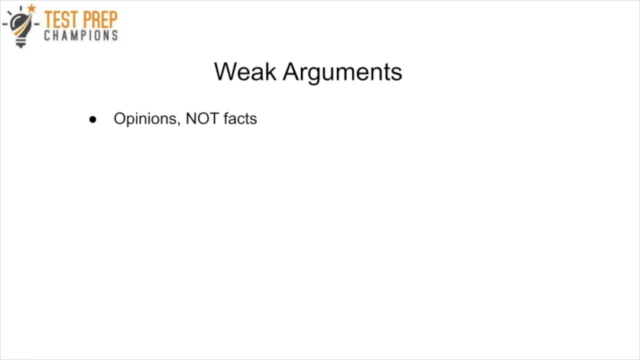 may be very credible, But if it's just the author or the person who's sharing their opinion, it's probably not credible. All right, also for unnamed experts, whenever someone is just saying: well, experts said this or experts said: 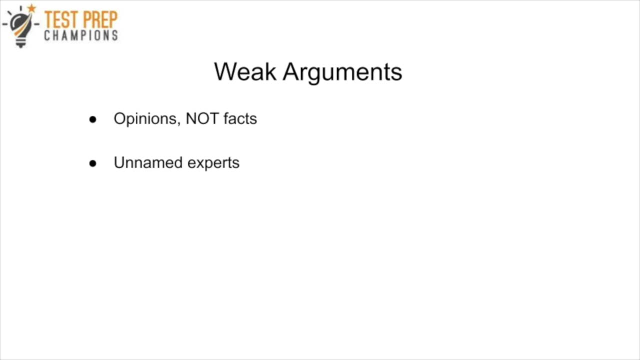 that, but they're not naming a specific expert or they're not including where they got the information. that's generally a sign of a weak argument. Also, any unnamed or unreliable sources, whenever somebody makes a claim in a piece but they don't state evidence or they don't state. 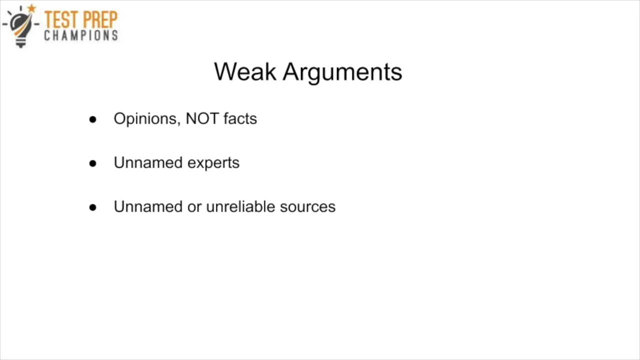 their data saying why they believe that. well, that's generally a sign of a weaker argument. Also, outdated sources, very older sources, generally make the argument less credible. And lastly, bandwagon And bandwagon- you can think of this as people just jumping on the bandwagon. 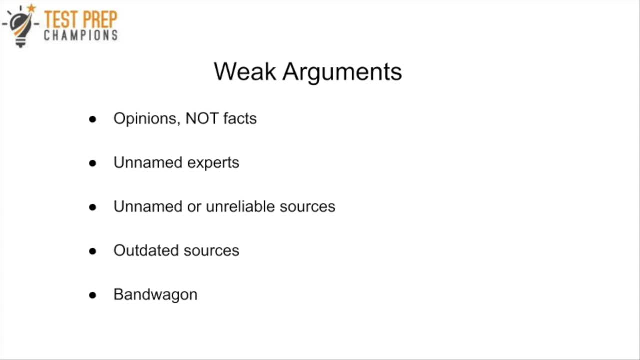 where if an author says: well, everybody's doing this or everybody knows that, well, those words are very, very strong, and it's rarely true in life that everybody believes something or everybody feels something, So that's a sign of a weak argument. Let's look at an example of this. 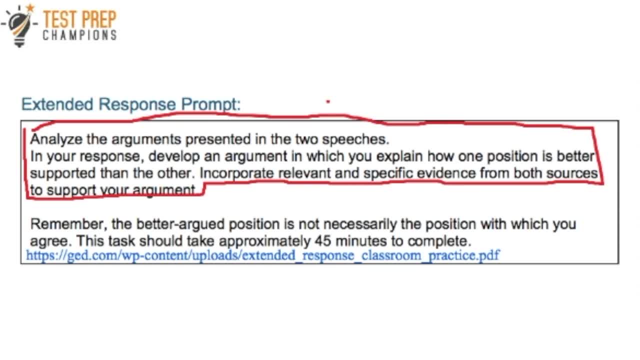 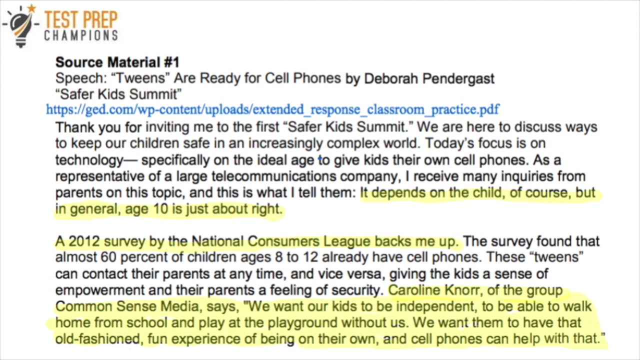 and here's the prompt. The prompt says So here. I've given you a snippet from the first passage here and, if you want to, you can pause the video and you can read this, or you can put the link that I've 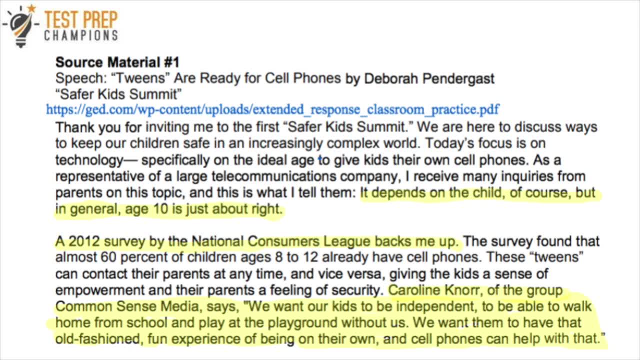 included here in your search engine. I'll also put this link down below, but that's not really that important for you to read the whole thing here. I just want to highlight a couple things here, and then we're also going to look at a second passage. So the first thing that you need: 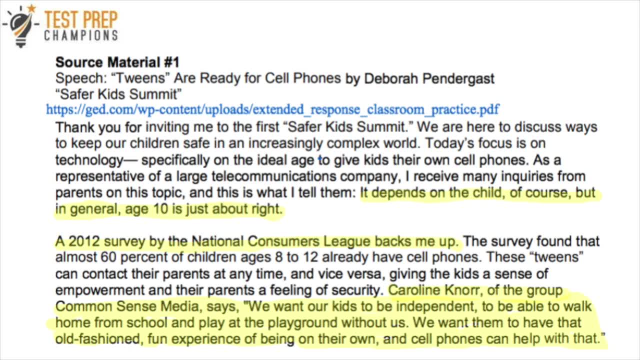 to know here, though, is that the two authors are arguing over the proper age for a child to get a cell phone at, And so I've highlighted here Deborah's position, and you always want to try to find the author's position right away whenever you're trying to read through your essay and plan. 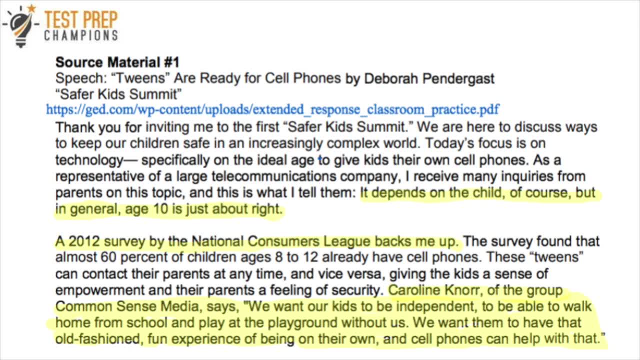 out what you're going to write. So here her position is: It depends on the child, of course, but in general, age 10 is just about right. So she thinks that, or she's trying to argue that 10 is about the right age to give a child a cell phone. 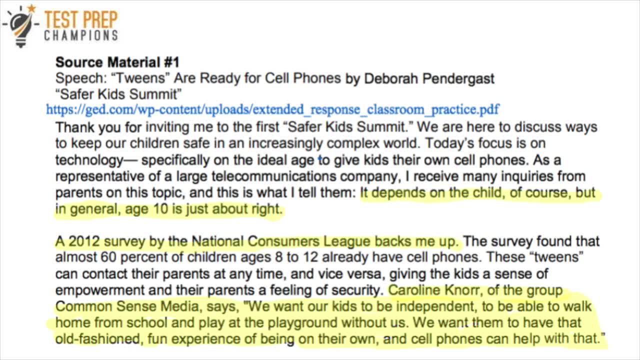 So what kind of evidence does she bring to the table here to support that argument? Well, we see here that she is citing from a survey done by the National Consumer League, and it was done in 2012,, which makes it a fairly recent survey. And we also see that she is quoting. 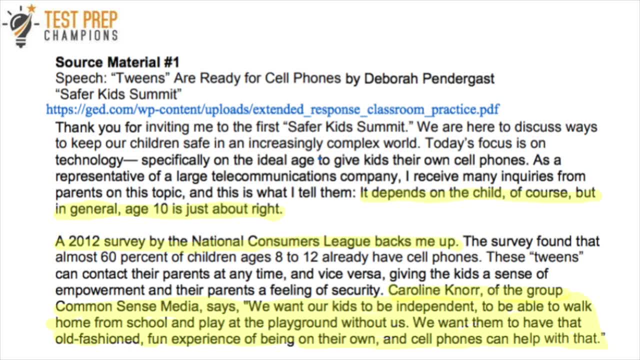 from an authority figure who is Carolyn Knorr, and she uses this quote in her article, and Carolyn Knorr is basically saying that we want our kids to be independent, and so giving them a cell phone is a good way to help them with that. 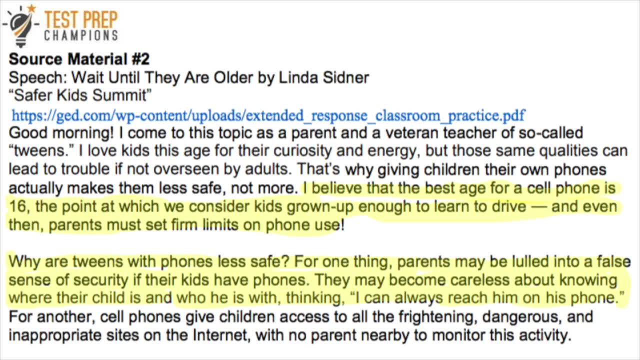 So now we're going to look at the other essay here, and in this essay the author is arguing that the best age to get a cell phone is 16.. So her purpose can be identified here, or her position, I should say, where she says: I believe that the best age for a cell 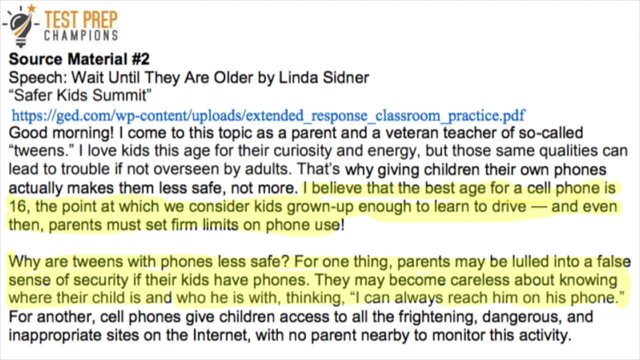 phone is 16, the point at which we consider kids grown up enough to learn to drive, and even then parents must set firm limits on phone use. So right off the bat we see that her position is 16, versus the other author who thought that 10 was the best age, or around 10 anyway. 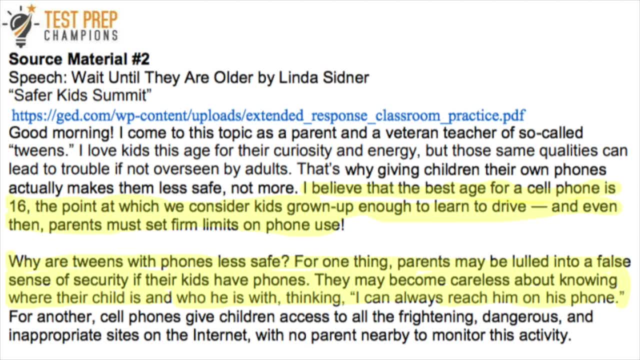 So what I want you to note here is a couple of things. First of all, she uses the words I believe, So I believe basically tells us that she's going to be giving an opinion here. She also says that even then, parents must set firm. 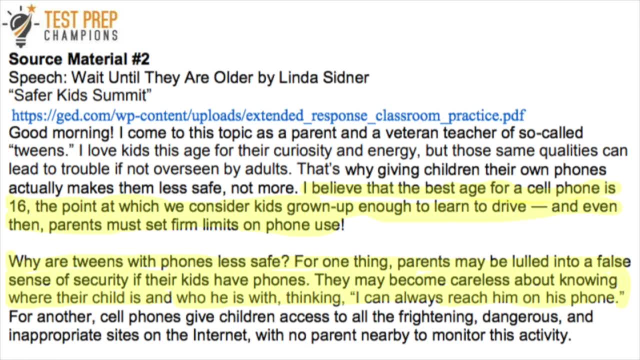 limits on phone use. And now, maybe you agree with that, maybe you disagree with that, but the point I want to make here is that she's not making any kind of facts or evidence for why parents must set firm limits on phone use. She's basically just giving her opinion. 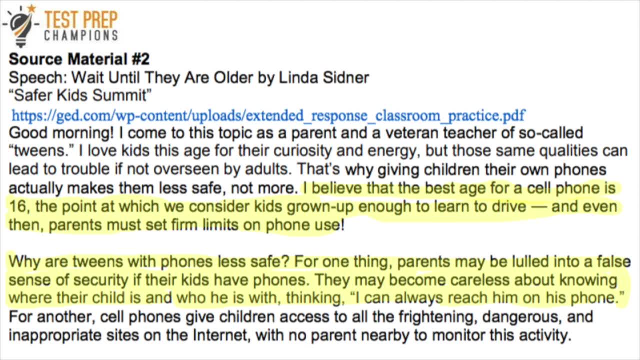 here She's making a claim without evidence. So she goes on to say: why are tweens with phones less safe? For one thing, parents may be lulled into a false sense of security If their kids have phones. they may become careless about knowing where the child is and who he is with. 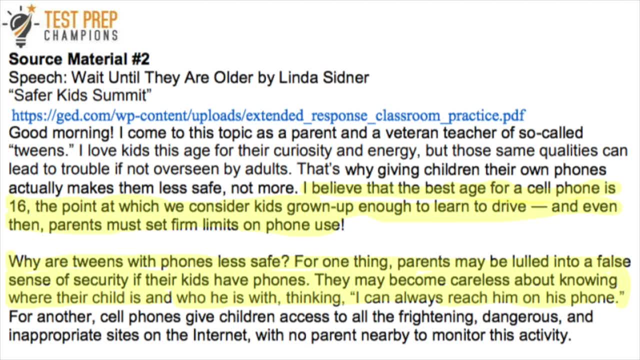 thinking: oh, I can always reach him on his phone. And now the point again here that I want to make is that she might be raising some good points here, So maybe you do agree with her on a personal level, but since she's missing facts and evidence data, she's missing results from surveys There. 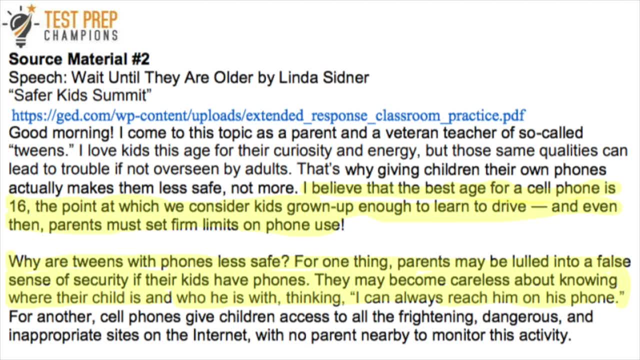 are no authority quotes or quotes from experts here that we can see. So, unfortunately, even if you agree with the points that she's making, we would want to consider this to be the weaker essay, based just off of the first little snippets that I'm showing you here. And again, the reason: 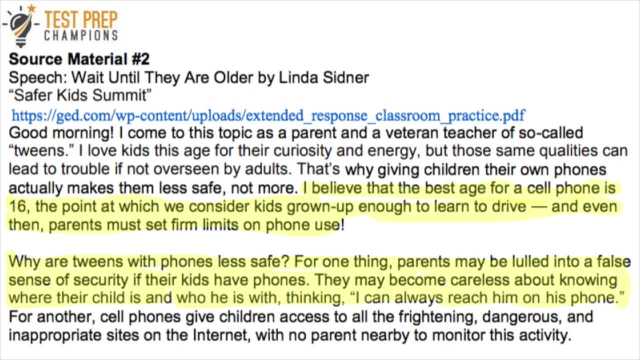 is because, while she may be making some interesting points here, some that you might agree with, at the end of the day she's not giving us facts or statistics or really any kind of evidence for why these claims make 16 the better age. So we would have to consider this: the weaker 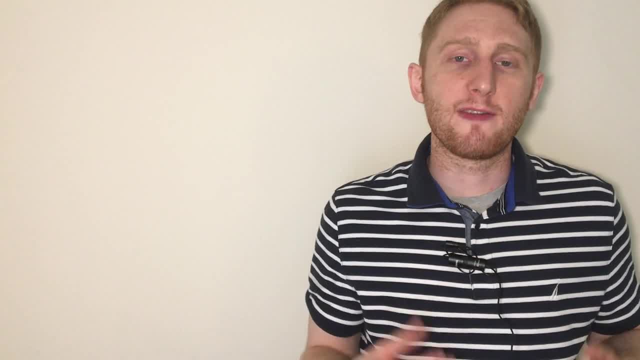 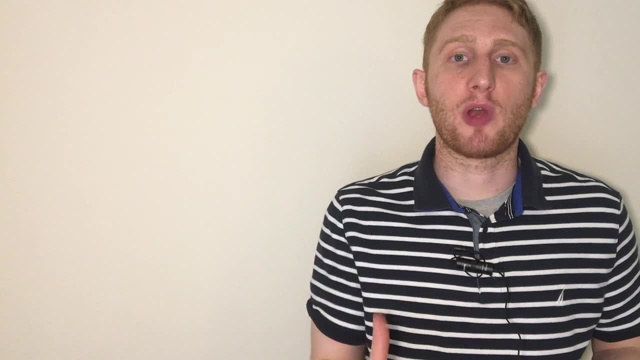 argument. So now I'm going to give you a formula or a format that you can follow when you write your essay, And this isn't something that I've made up, But this is a great structure that will really help you with your writing process, And it's called the five paragraph essay. Basically, how it works is you'll. 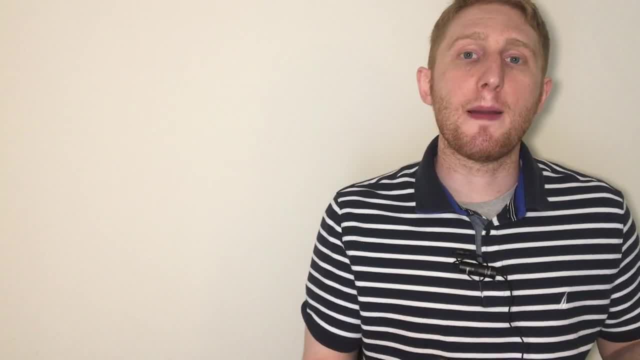 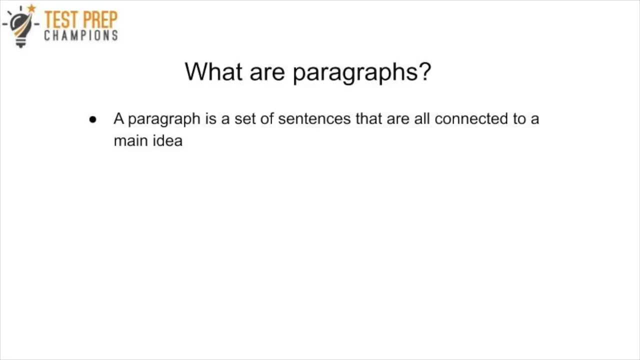 start off with an introduction paragraph. then you'll have three body paragraphs that are going to make up the bulk of your essay. then you'll end with a brief conclusion. Now let's go more in depth here on how exactly to do a five paragraph essay. So, first of all, what are paragraphs? Well, 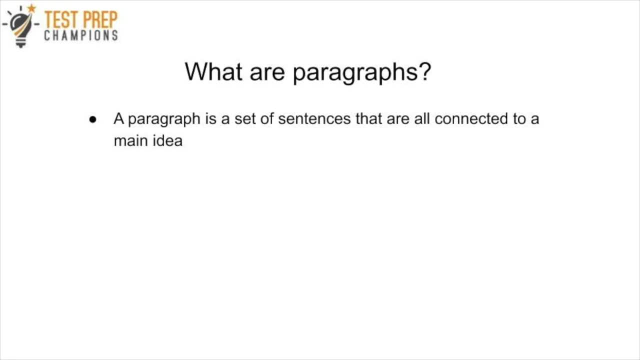 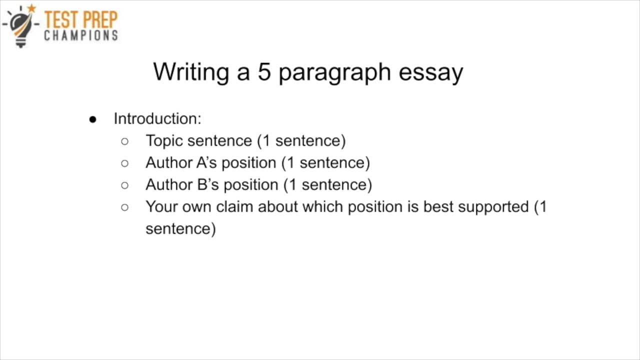 a paragraph is just a set of sentences that are all connected to a central idea, And when you write a five paragraph essay, this is a great formula to use for your introduction here. So you'll start off with a topic sentence, which is just one sentence. then you'll state author A's position. 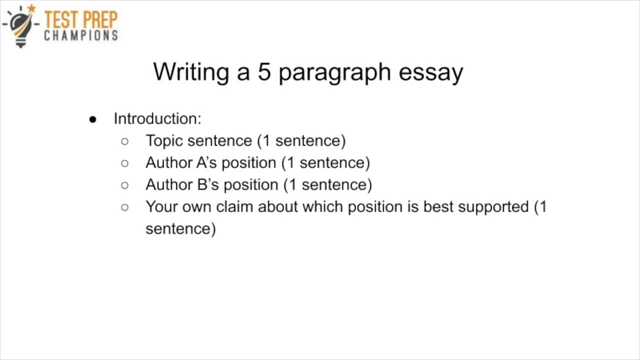 and then the other author's position And then, lastly, you'll put one sentence that is your own claim about which position is best supported by the evidence in the text. And now, this is not the only way to do it. There are other ways that you can do it. There are other totally valid ways. 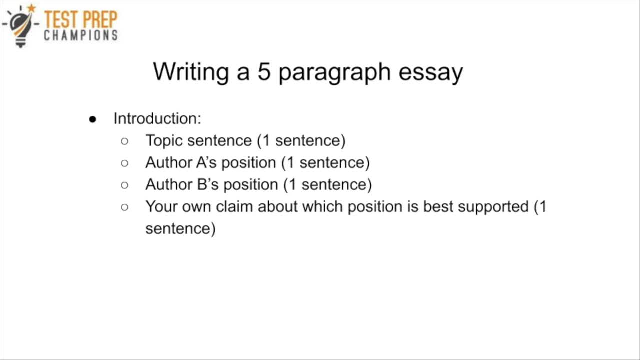 to do it, But this is the way that I recommend doing it. This is a good approach to maximize your points And it's just kind of like a formula that you can use here. And so let me give you an example here, And this comes right out of those cell phone passages. So your topic sentence is: 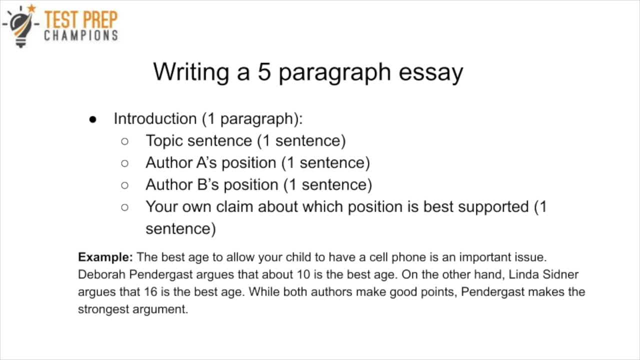 just kind of a sentence that just introduces the topic at hand. It doesn't necessarily say anything about which author's position you thought was stronger, It's just introducing the topic. So I said the best age to allow your children to have a cell phone is an important 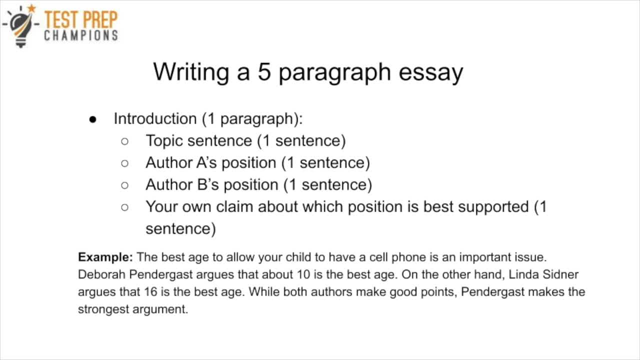 issue. Nothing fancy just gets the job done here right. So that's the way that I recommend doing it. That's would be my topic sentence. And then the next sentence that I wrote is that Deborah Pendergast argues that about 10 is the best age. So I'm just stating the first author's position. 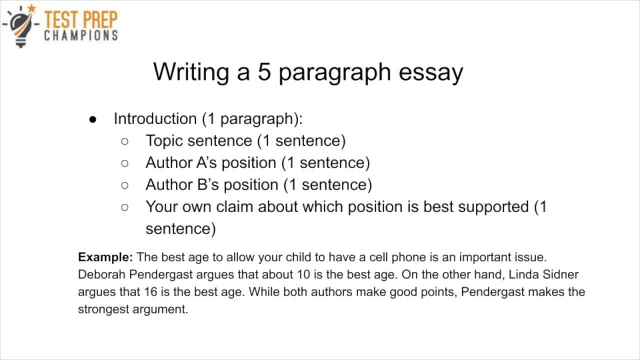 here. Then I state the second author's position And I say: on the other hand, Linda Sidner argues that 16 is the best age. And then, lastly, I end the introductory paragraph with a claim about which position I believe is best supported. So I say, while both authors make good points, 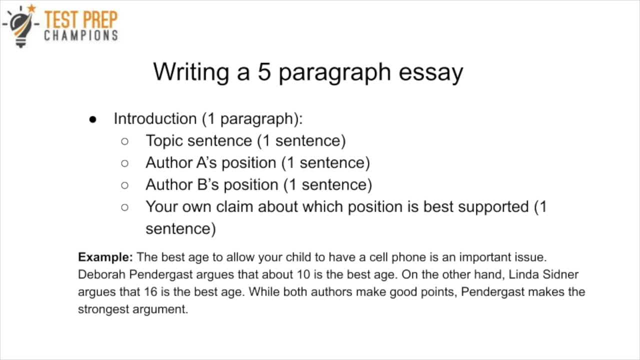 Pendergast makes the strongest argument. All right, And so again, you know, this is just an example I made up off the top of my head, just to drive the points home here. This isn't necessarily the best way to possibly write an essay about this, You know. 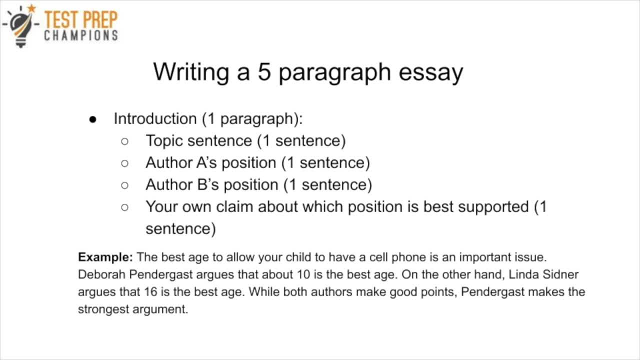 I wasn't trying to win any awards with my essay writing skills here. I just wanted to give you an example of a totally valid way to do it where it's just a formulaic approach. Just come up with a topic sentence that's something relevant to the topic being discussed, to show that you know what. 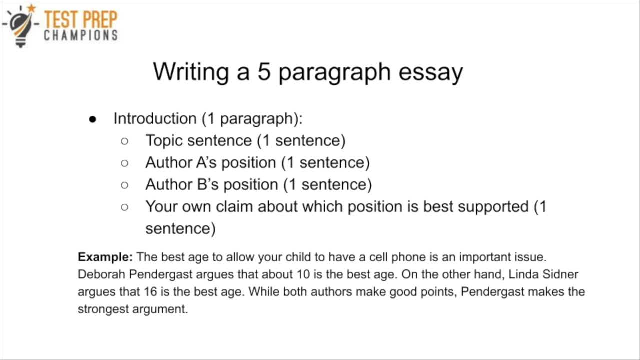 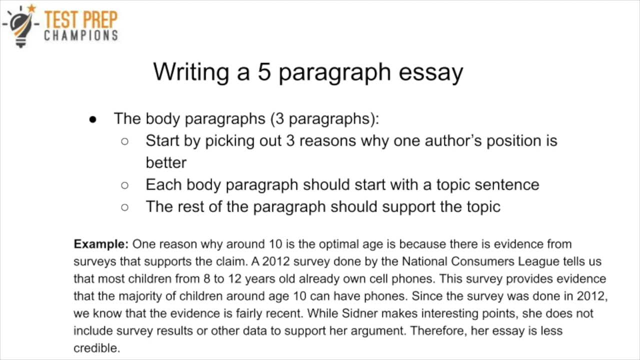 the topic is: Introduce both authors' positions and make the claim about which position you think is best supported, And then keep moving. Just keep it simple. So then next, what you want to do here is for your body paragraphs. remember, you're going to have three different body. 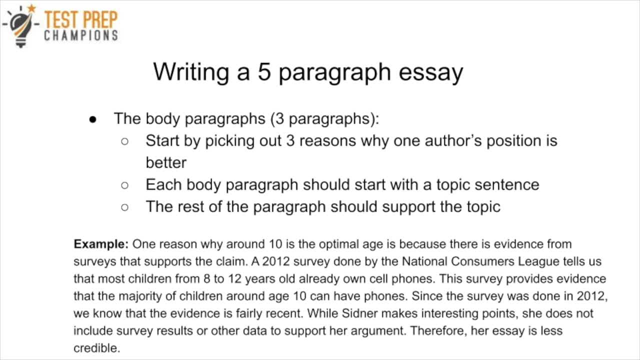 paragraphs. Okay, And you're going to start off by picking out three reasons why one author's position is better. So, during your planning, I want you to think about you know three, at least three different reasons why the author's position is better than the others. Okay, And they? 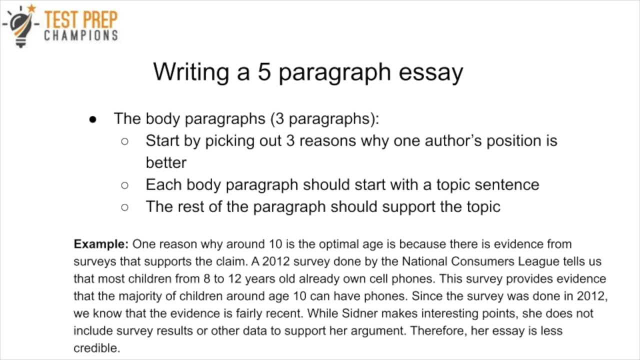 could also be reasons why an author's position is weaker. All right, And so each body paragraph is going to start off with a topic sentence, And then the topic sentence is going to be a topic sentence, And that's going to basically be why you think one of those three reasons makes the gives better. 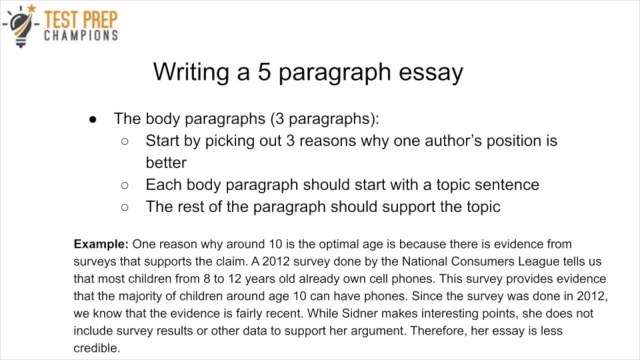 evidence for the author's position. Okay, And the rest of the paragraph is then going to support that topic sentence. So I know that this kind of sounds a little bit confusing, but let me show you an example here. So let's say that again. here was my introductory paragraph and here's my example. 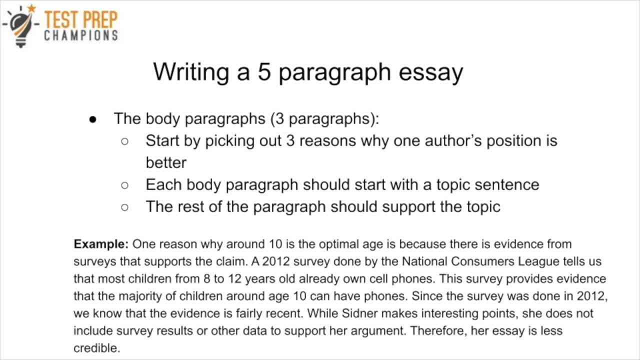 for my introduction. Then here this is an example of how I could write a body paragraph. So my topic sentence would be: one reason why around 10 is the optimal age is because there's evidence from surveys that supports the claim, And so that would be my topic sentence. And then the topic sentence. 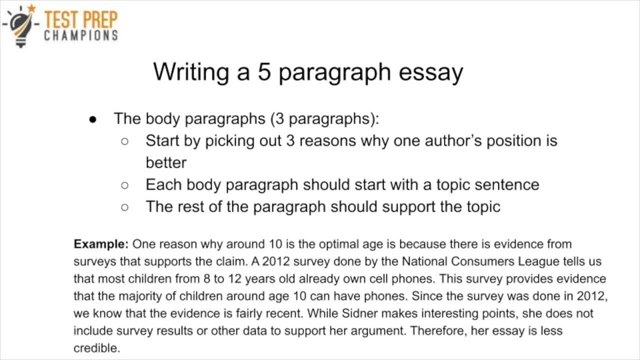 I'm just picking one reason why I think that author's position is better here. It's because there's evidence from a survey that supports the claim. And then I'm just using the rest of the paragraph to explain what I mean by that, using the evidence from the text. So I go on to say: 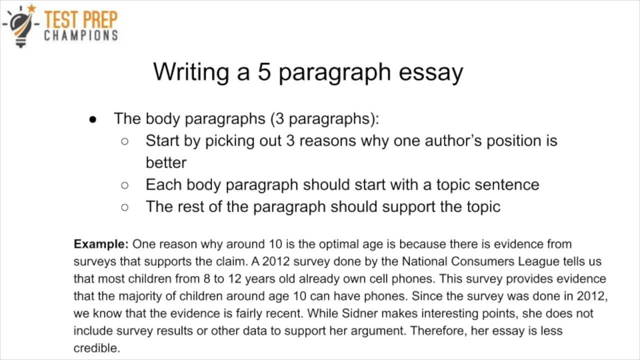 a 2012 survey done by the national consumers league tells us that most children from eight to 12 years old already own cell phones. This survey provides evidence that the majority of children around age 10 can have phones. Since the survey was done in 2012,, we know that the 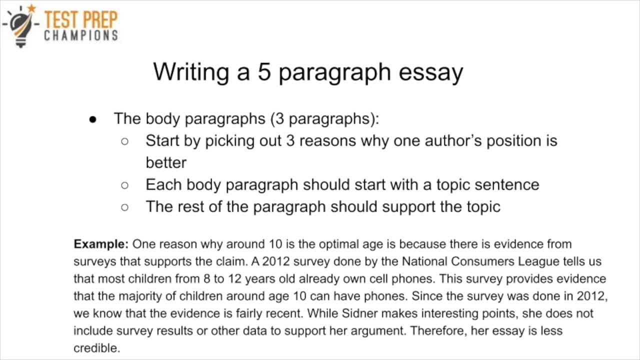 evidence is fairly recent. While Sidner makes interesting points, she does not include survey results or other data to support her arguments. Therefore her essay is less credible. All right, And so again, you know, this isn't necessarily the ultimate or the best. 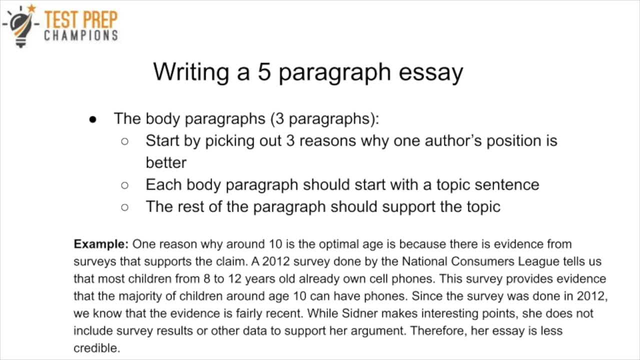 way to write this essay by any means. I just put this down as an example, But this is just a totally valid way of doing it, where I'm just picking out one reason why I think that this author is right, And so then I just basically explained that in the paragraph, And the reason I picked was because 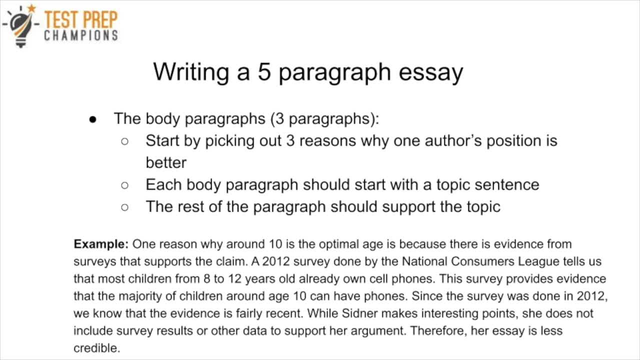 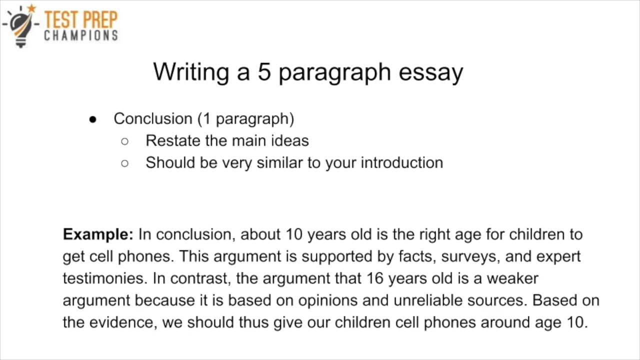 she uses evidence from a survey, And I just explained why that makes her case stronger and why the other person argument was weaker because her essay was less credible and didn't have these results in it from surveys. All right, so your conclusion is really, then, the simplest part. It's basically: you're just 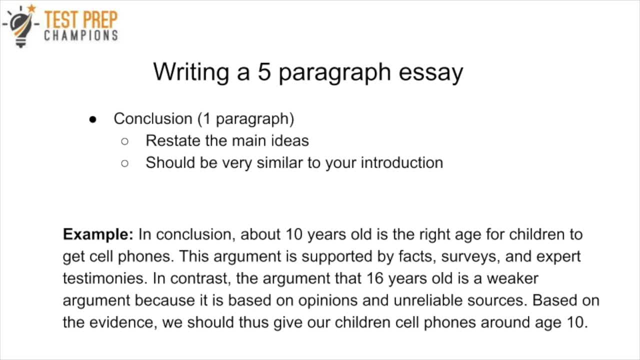 restating the main ideas, and it should be very similar to your introduction. It shouldn't take you that long. So basically, you can always just start by saying any conclusion, And so in my example here I say a conclusion about 10 years old is the right age for children to get cell phones. 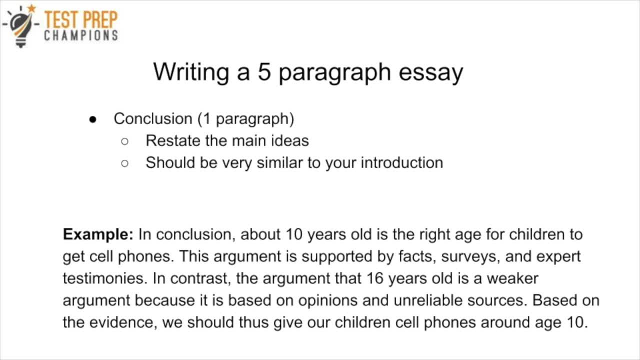 This argument is supported by facts, surveys and expert testimonies. In contrast, the argument that 10 years old is weaker is a weaker argument because it is based on opinions and unreliable sources Based on the evidence. we should thus give our children cell phones around age 10.. Okay, 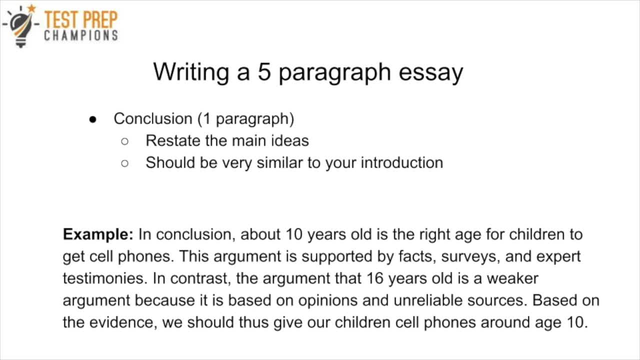 and so I didn't show you two examples of two other paragraphs for the body. So just note that I only showed you one example of a body paragraph because I don't want you to get bored to death because this isn't the most exciting topic. So know that you would want to do two more And again as 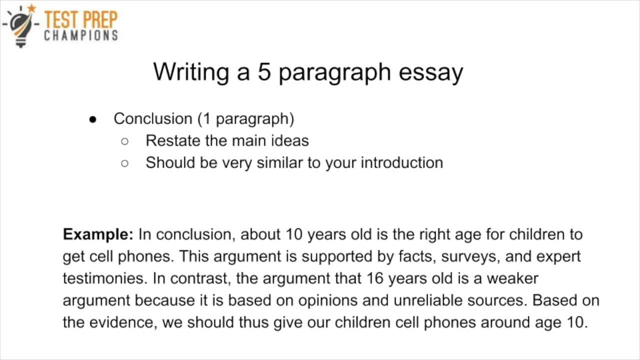 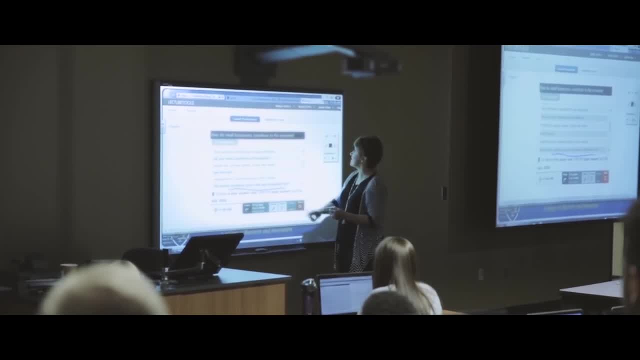 I've said it 10 times here. I'll probably say it another 10 times, Right? This isn't necessarily perfect way to do this essay. I just wanted to show you one example of how you can use this five paragraph essay approach to write your essays, And it's a totally valid approach to. 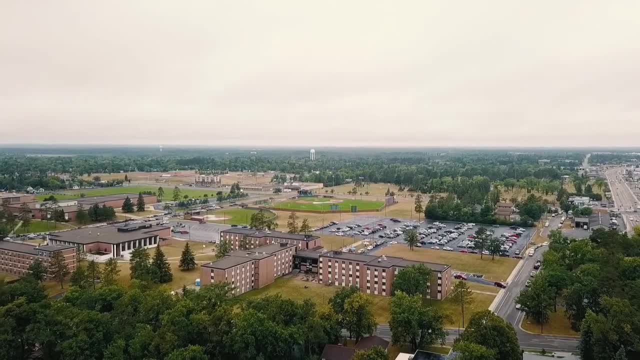 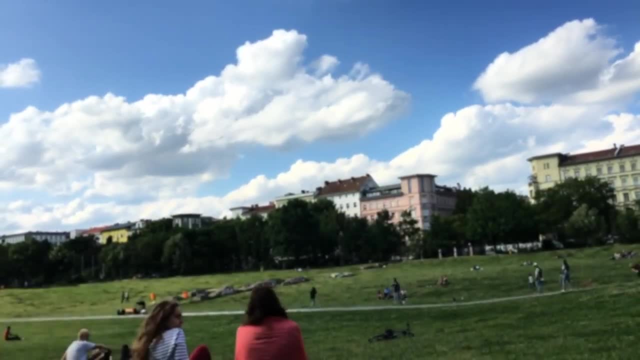 doing it. It's simple, It's to the point And really you know you're going to be graded on. is there a structure? Is there an organization? Is there a logic to your argument? And just by following this point, these points here about how to write the five paragraph essay, you know. 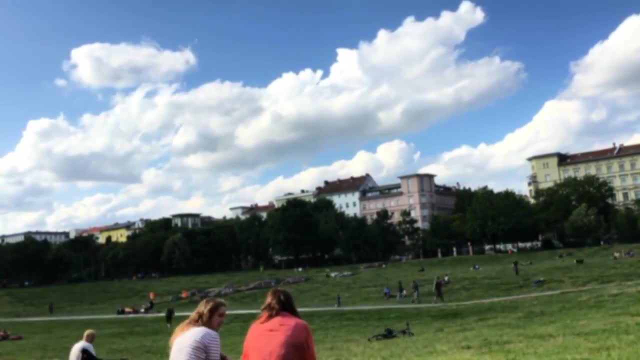 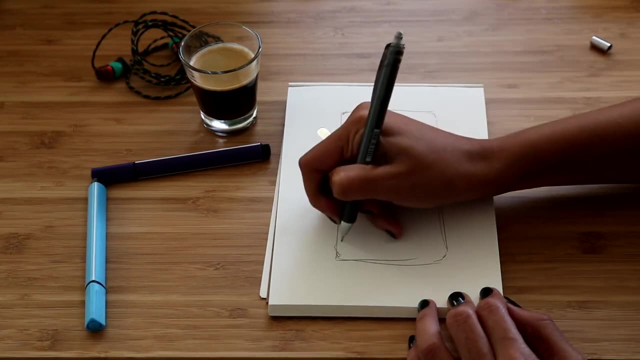 you just organize your thoughts here. Really, it really goes back to that planning. You want to do that planning so that you identify strong and weak points, so that when you go to write you already have a good idea of who is making the strongest argument. Okay, And then from there. 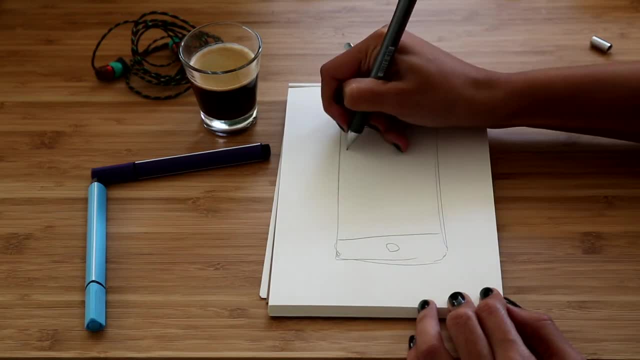 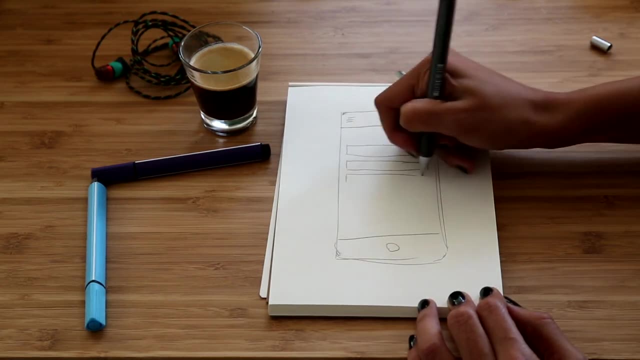 you're just going to organize this so that you pick out some reasons why you think that that person's argument is strongest, and that's going to be in your body, And then you know, put that intro and that conclusion and then you're done. That's really it. So after you finish your essay, 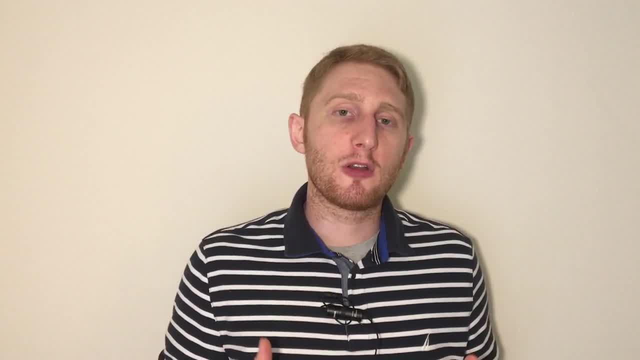 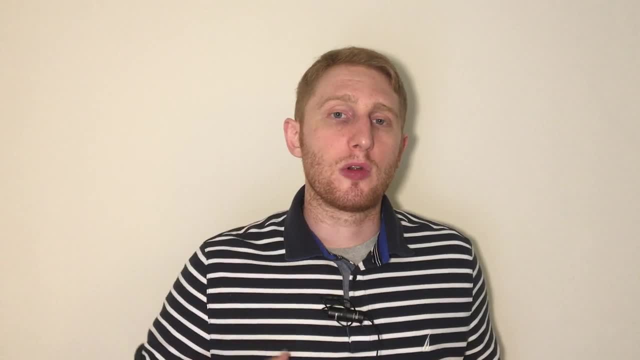 let's say you've got maybe five or 10 minutes left to check your work. You want to look for grammar mistakes as you're editing. You want to look for places where you're using periods or commas or questions. You want to look for things. like you know, you're writing a sentence. 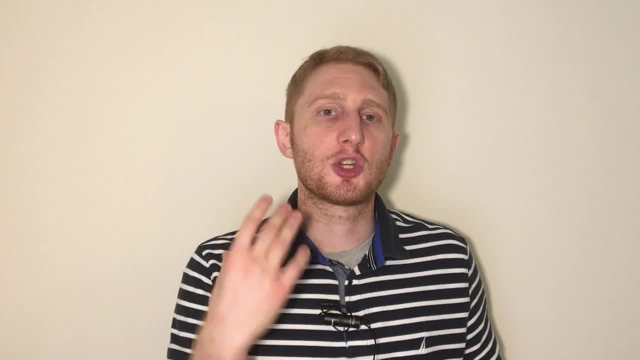 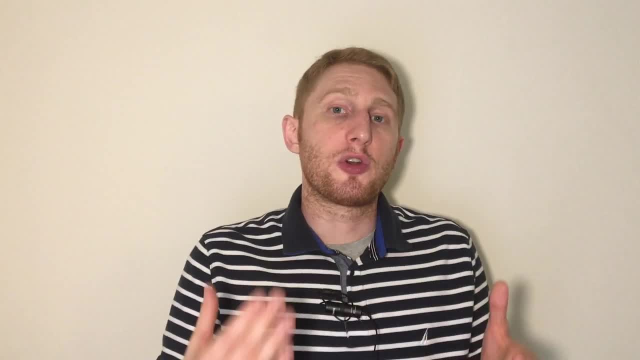 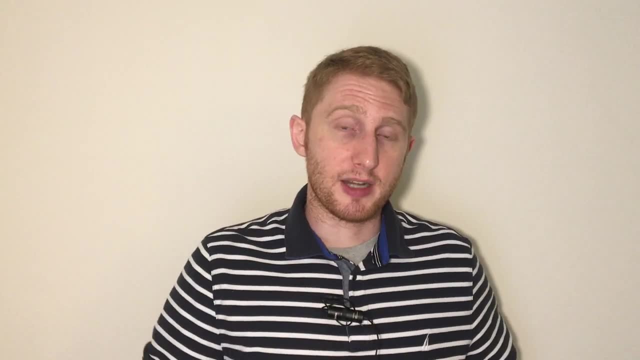 wordy and see if you can break a sentence into two shorter sentences. right, So take a long sentence and condense it into two shorter sentences. If you're using colons or semicolons, make sure that you're using those correctly. This is all stuff that I don't want to get into in this video here.